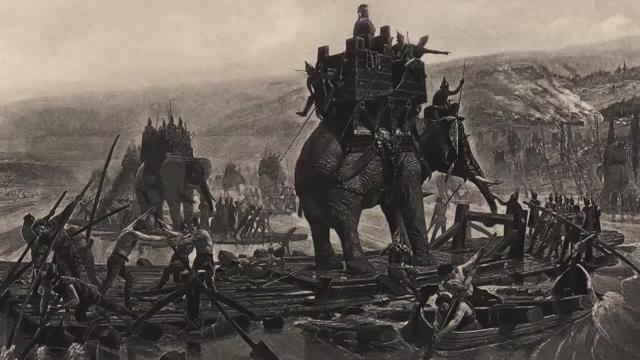 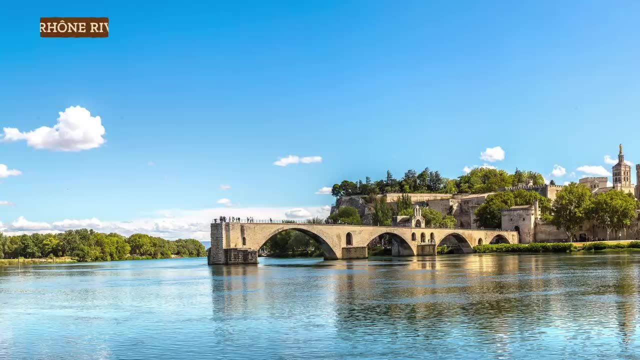 or gaining strategic control of mountain passes and rivers has often been the key to empire building. But we'll leave the plot of that story for world history. Today, we'll focus instead on the setting, the landscapes over which they traveled. The topography or shape of a region or land has influenced so much. 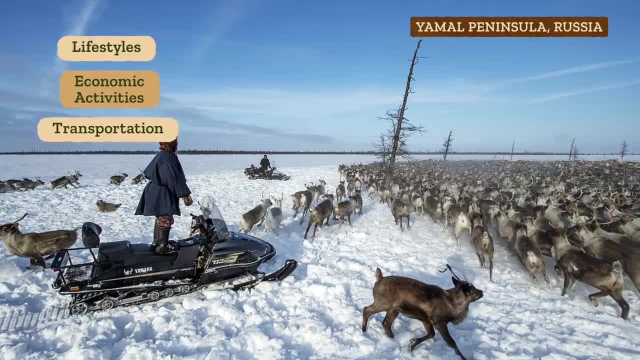 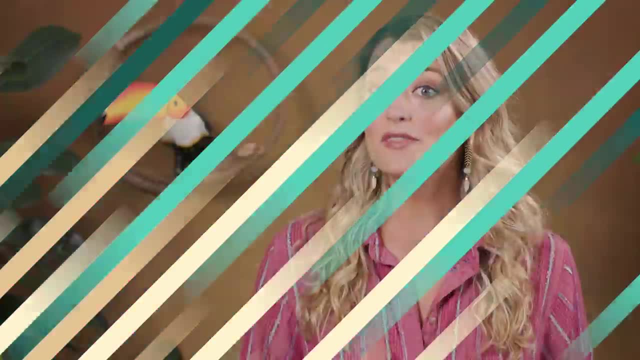 like lifestyles, economic activities and transportation. We've even gotten different cultures and languages thanks to isolated communities flourishing in places that are hard to access by the outside world. So, as physical geographers, we want to know how the scene the Earth was set. 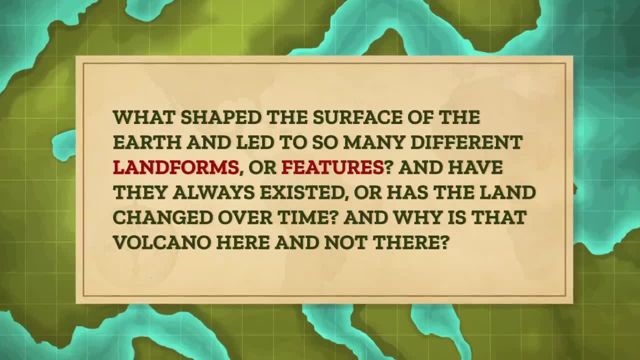 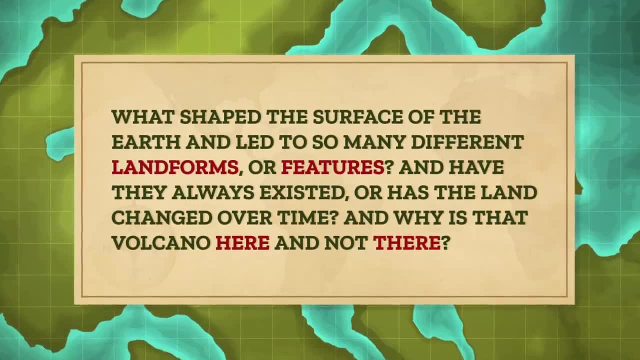 Like what shaped the surface of the Earth and led to so many different landforms or features, And have they always existed? or has the land changed over time? And why is that volcano here and not there? We already know the Earth is the result of many processes. 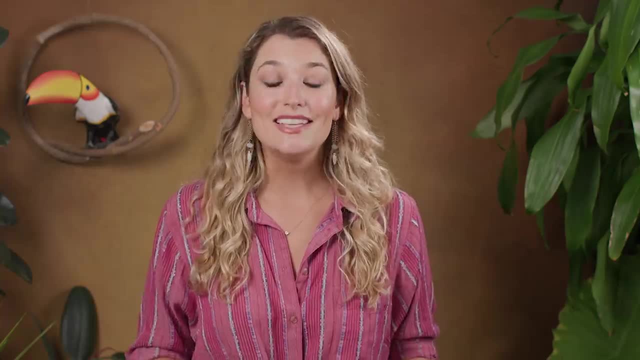 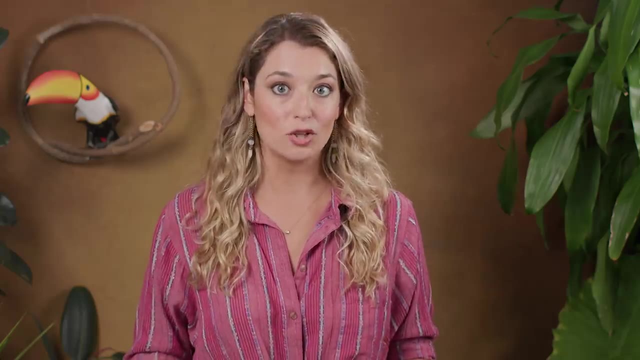 and its topography is no different. Some processes operate deep within the Earth's interior and some stay at the surface. But just as the atmosphere and biosphere are always changing with the flow of energy and cycle of nutrients, these processes in the lithosphere change the very ground beneath our feet. 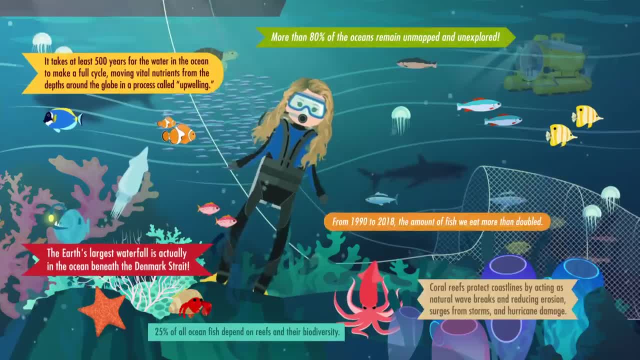 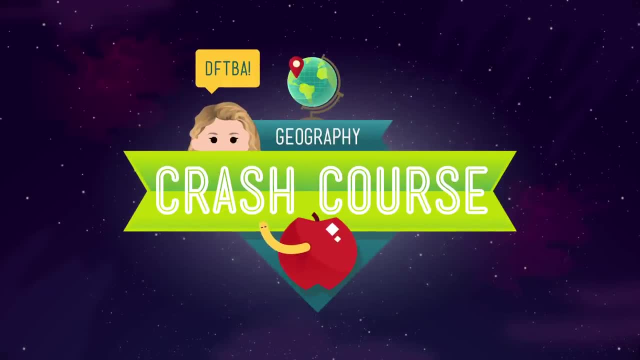 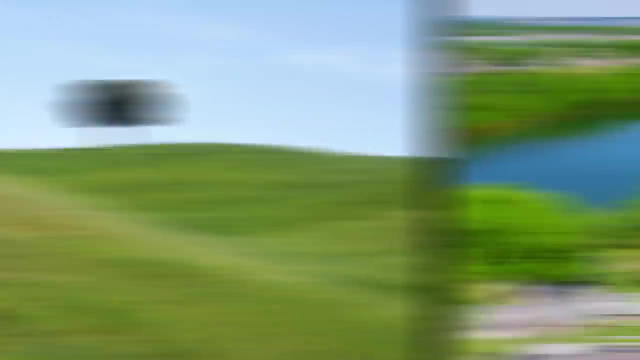 I'm Alizé Carrère, and this is Crash Course Geography. Whether we live in a city, a suburb or the countryside, we're embedded in particular landscapes. We see these hills or ponds or lakes every day, and they become ordinary to us. 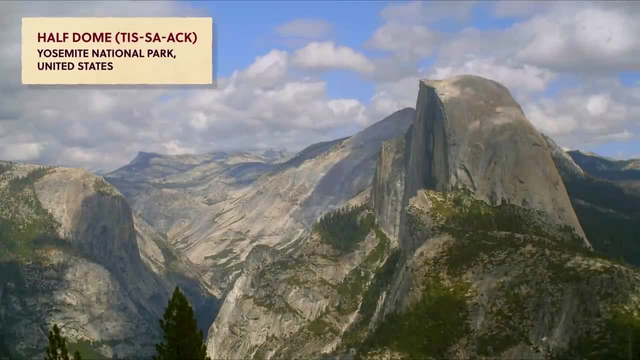 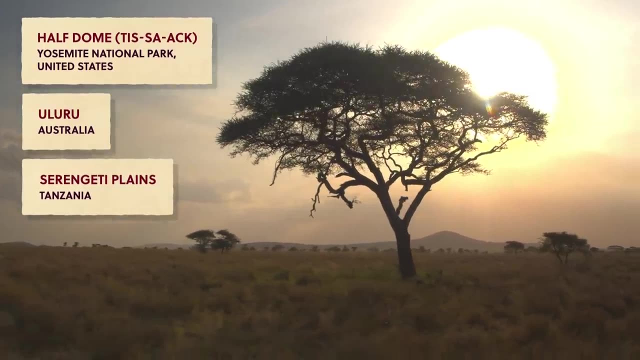 So we visit impressive landscapes like the places we now call Half Dome and Yosemite National Park in the US, Uluru in Australia or the Serengeti Plains in Tanzania- all natural environments that fill us with a sense of grandeur and awe. 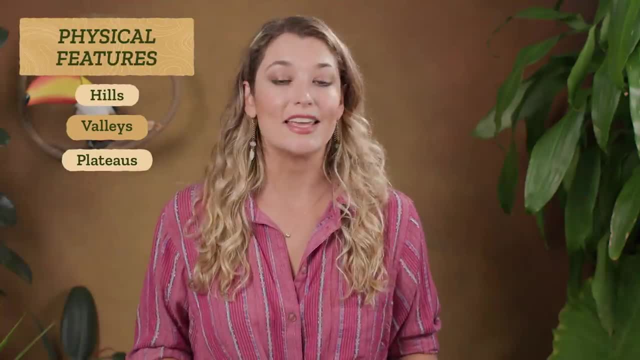 But no matter where we are, the land is made up of physical features like hills, valleys and plateaus, And we can study all these physical features, even the ordinary ones: Geomorphology in the Valley of the Sea and the Sun. ocean and earth are both the most important elements of genetic research. 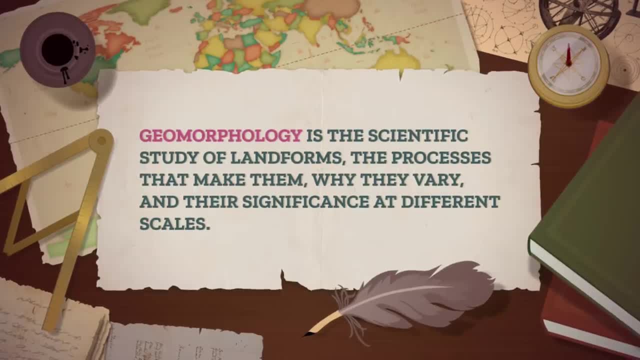 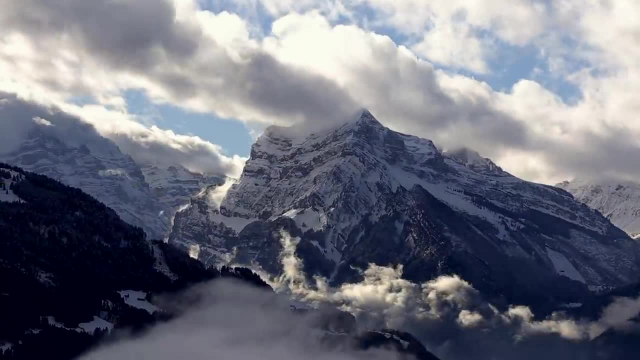 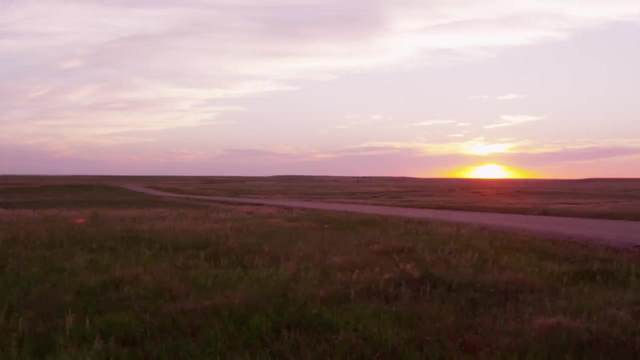 Geomorphology is the scientific study of landforms, the processes that make them, why they vary and their significance at different scales. Towering mountains or flat plains that stretch as far as the eye can see can seem timeless, but they're actually always changing, thanks to a network of intertwined systems that recycle. 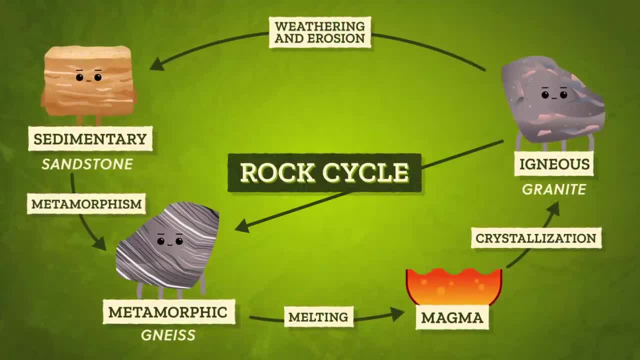 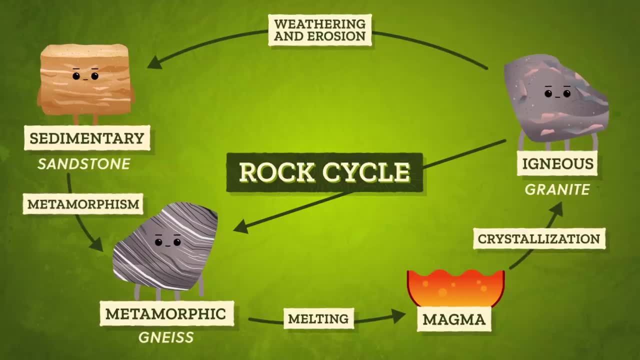 and reshape the Earth. Like the rock cycle moves minerals through igneous, sedimentary and metamorphic phases that shape much of the Earth's crust, and relies on processes both deep inside and on the surface of the Earth, And where those rock cycle processes are forming and destroying rocks follows a pattern we 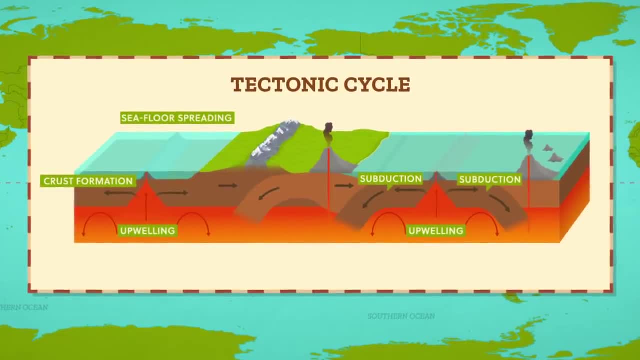 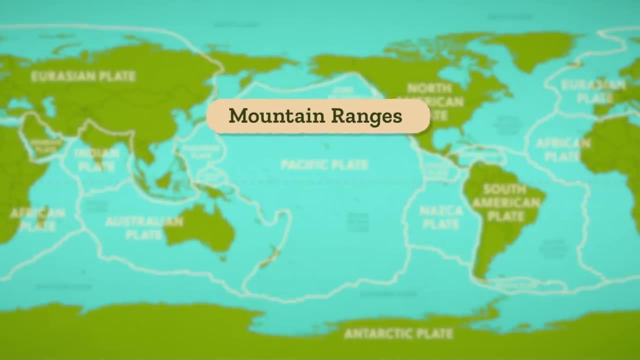 call the tectonic cycle. The tectonic cycle works on a huge scale and moves vast sections of Earth's crust, called plates, around the globe, which creates major geographic features like mountain ranges, ocean basins and continental shields. And there's the hydrological cycle, which explains how water is continually transferred. 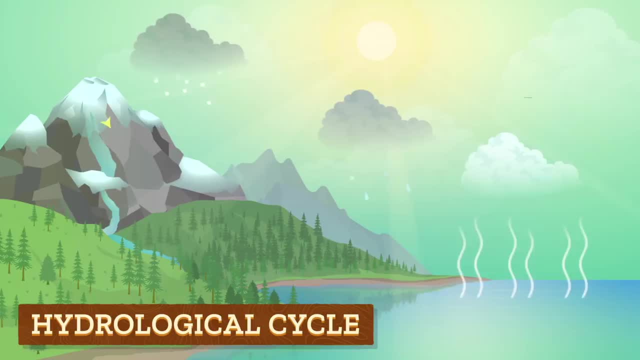 between being liquid, gas or solid, as it circulates into and out of the atmosphere, lithosphere, hydrosphere and biosphere, each of which is its own system where it moves into and out of the atmosphere, lithosphere, hydrosphere and biosphere. 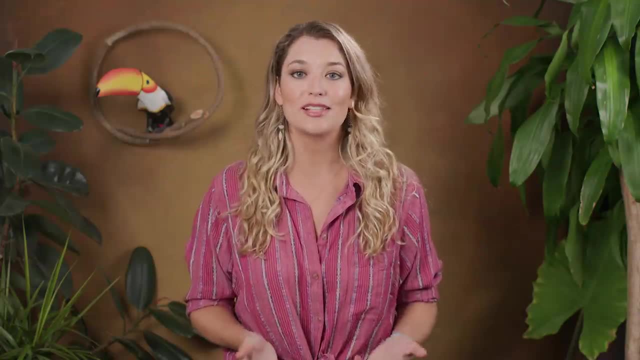 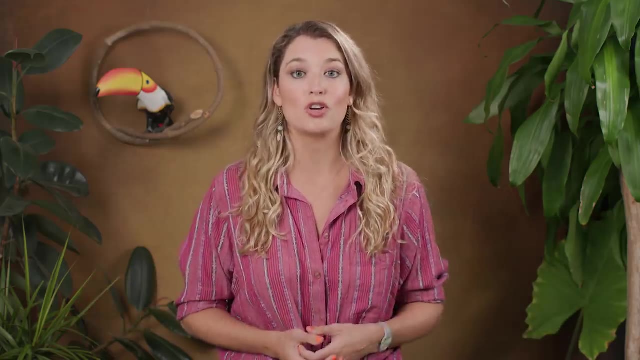 with numerous subsystems. The rock, tectonic and hydrological cycles and their many subsystems make up the geological cycle. They also showcase the give and take between two overarching internal and external systems that shape the topography where Earth, atmosphere and ocean all come together. 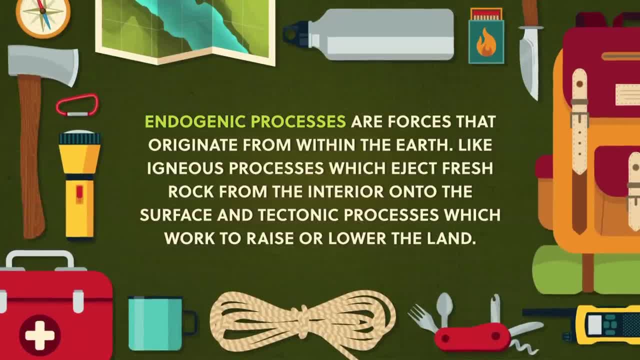 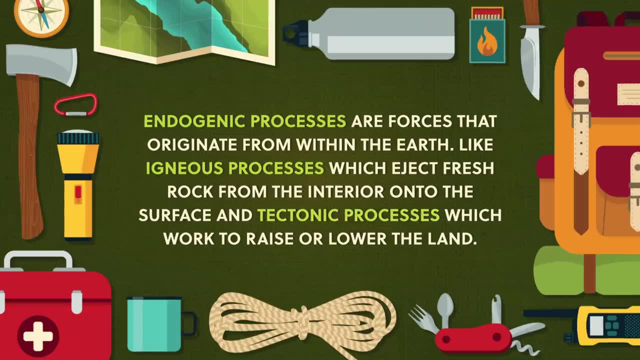 endogenic and exogenic processes. Endogenic processes are forces that originate from within the Earth, like igneous processes which eject fresh rock from the interior onto the surface, and tectonic processes which work to raise or lower the land. They produce initial landforms, kind of like the first broad strokes in a painting. 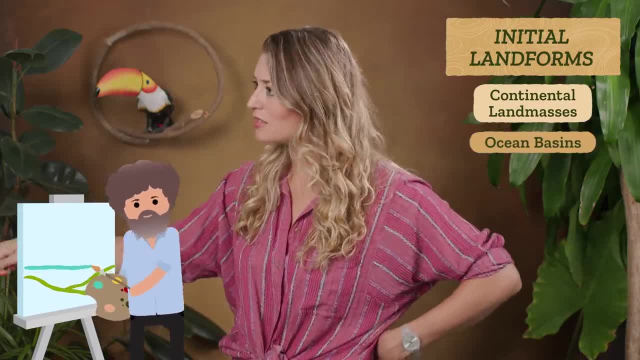 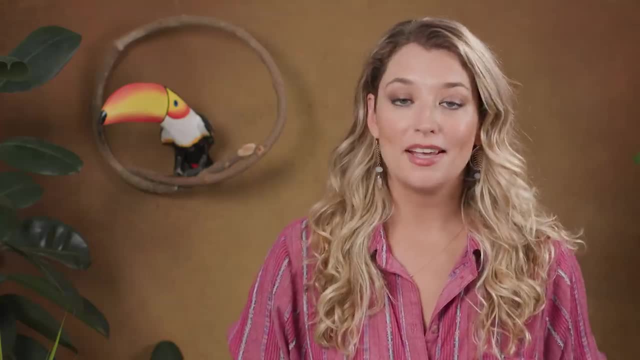 Like continental landmasses, ocean basins, mountain ranges that span across entire continents- The fine details will come later- To create landforms from igneous and tectonic activity. the rock cycle, the tectonic cycle and the hydrological cycle trigger each other. 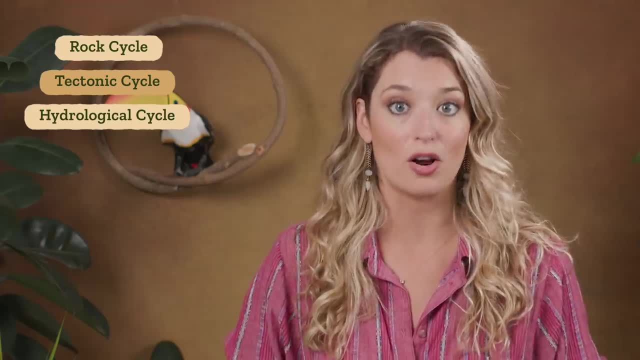 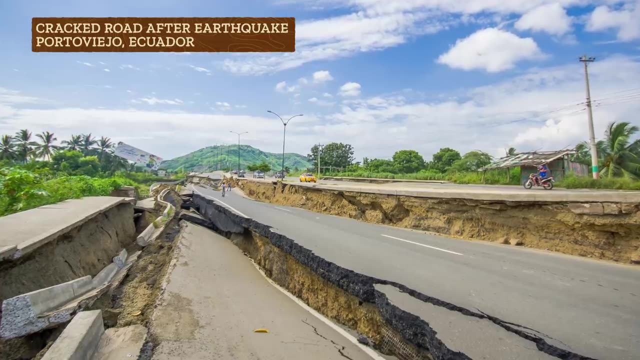 above and below ground in a variety of ways that change the topography. The powerful forces unleashed by tectonic activity as plates shift around the globe and cause earthquakes and tsunamis put rocks under tremendous stress, and rocks respond to stress differently. 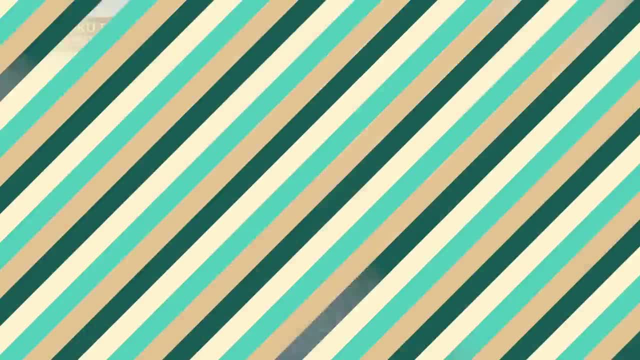 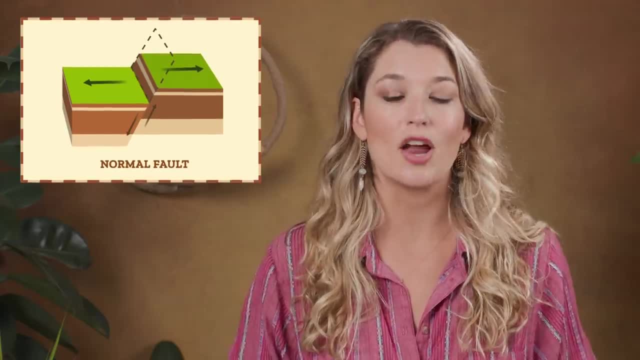 depending on whether they're on the surface or buried deep down. Rocks at the surface are brittle and when tensional forces from moving plates pull the crust in different directions, they come under stress or pressure and break or fracture in a process called faulting. 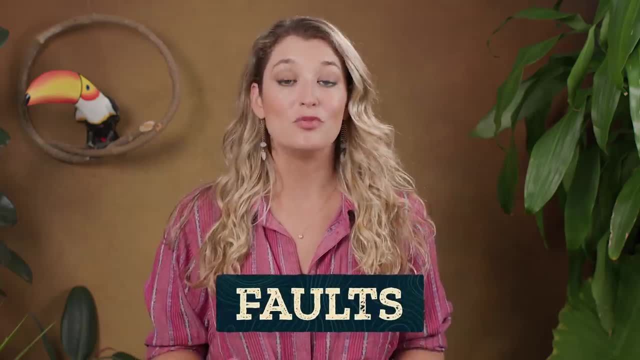 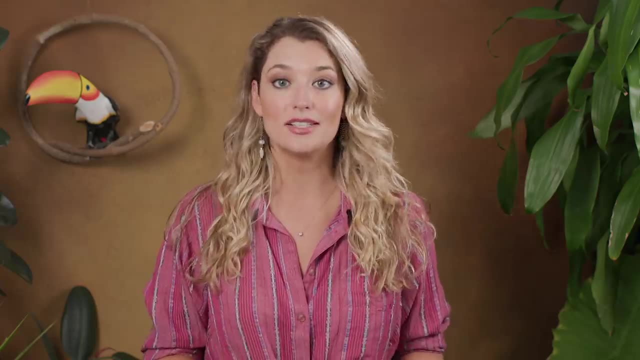 These cracks or faults in the Earth's crust show how the rock has moved on either side. The rock might have moved, horizontally or vertically, as little as a centimeter or up to 15 meters over years, decades or centuries. Like in September 2005,, a series of earthquakes occurred along a segment of what's called the 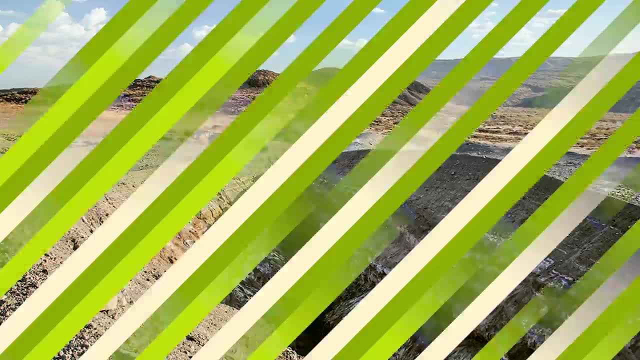 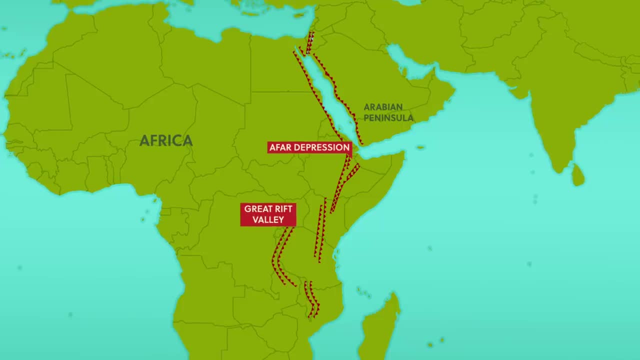 Afar Depression, creating an opening 8 meters wide, Though this was nothing new for the region, because the Afar Depression is an area of open fissures and faults at the northern tip of the Great Rift Valley, And the Great Rift Valley is a primary branch of the East African Rift System. 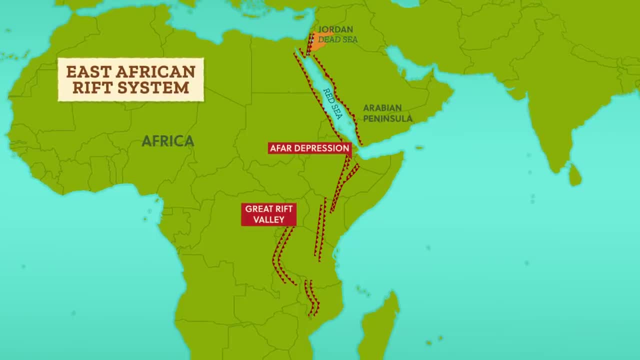 which extends from present-day Jordan in the north, through the Dead Sea and the Red Sea and along the length of East Africa to the mouth of the Zambezi River, Kind of like how the volcanoes of the Ring of Fire mark the plate boundaries of the 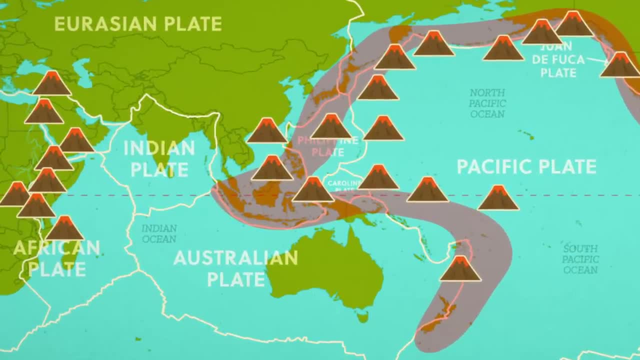 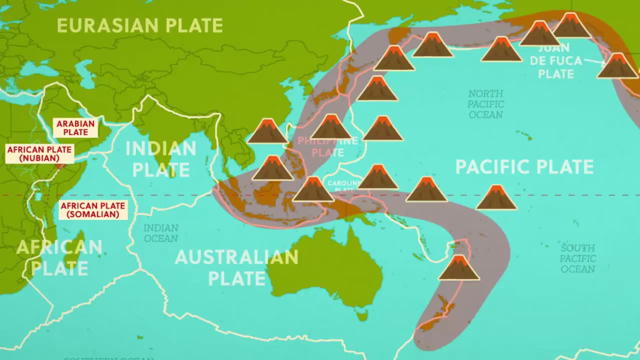 Pacific Ocean. the East Africa Rift System lies along the boundaries of three tectonic plates: The Arabian, African Nubian and the African Somalian plates. It's a huge set of faults that started to form when the plates began to diverge- about 25 million. 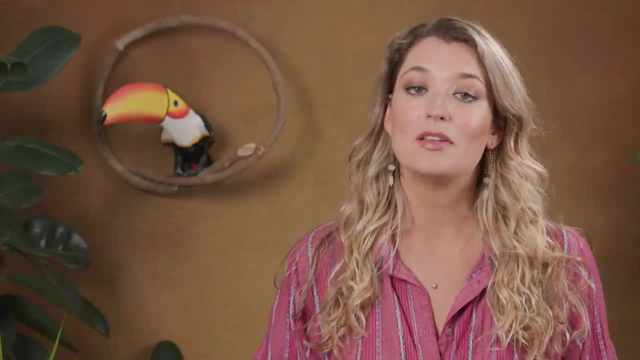 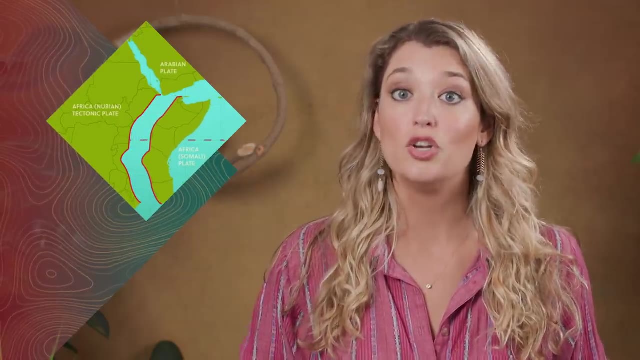 years ago. The Sudden Rift in 2005 was just a small step in the long process currently tearing the northeast of Ethiopia and Eritrea from the rest of Africa. Eventually it will create a new ocean, But that will take millions of years. 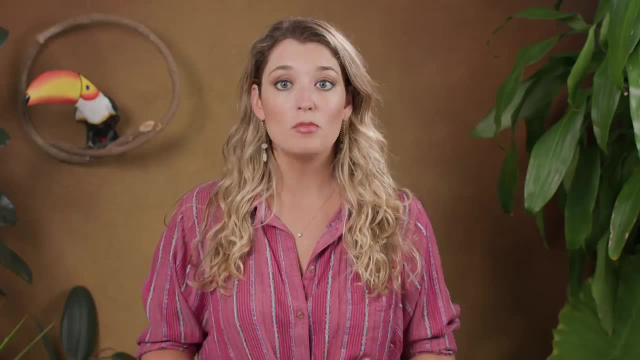 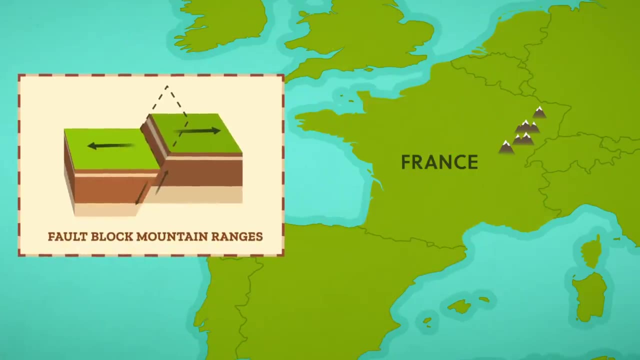 In particular, some of the faults of the East African Rift System are normal faults, a common type of fault created where the crust is moving apart vertically On a grand scale. when pairs of faults work together, they produce block or fault-block mountain ranges like the Vosges in France. 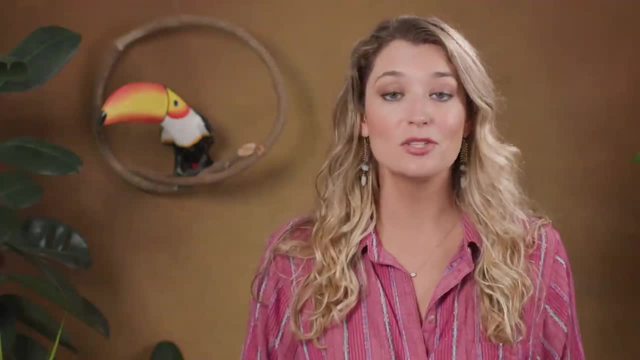 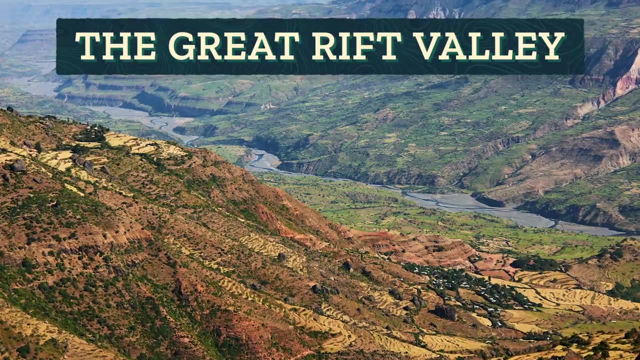 Though faults and fissures, and the volcanic and earthquake activity that comes along with them, haven't prevented humans from living on the edge, Tectonic clashes in the Great Rift Valley have carried on for tens of millions of years, But just a few million years ago, the journey of human evolution was recorded in the sediments and 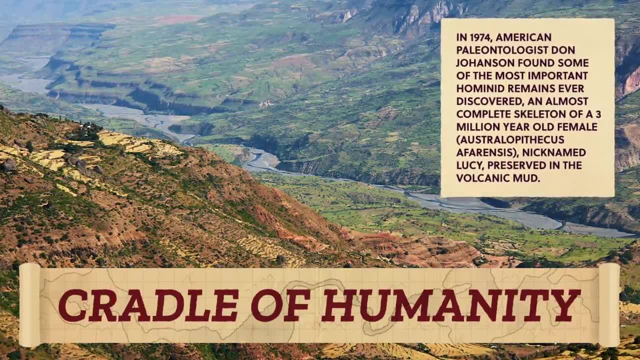 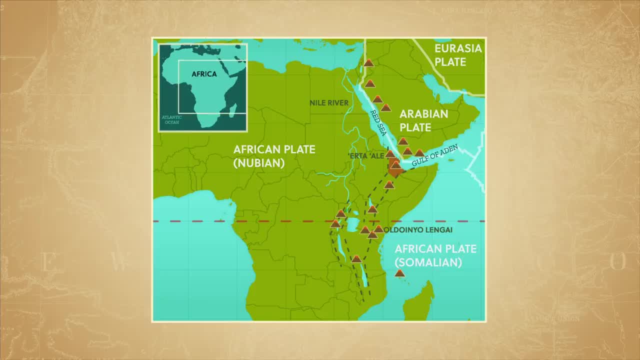 fossils throughout the region that some call the Cradle of Humanity, as our early pre-human ancestors walked and climbed across these valleys. Today, the fertile slopes of the many volcanoes that dot the length of the rift and the deep, elongated lakes on the valley floor are home not only to wildebeest giraffes. 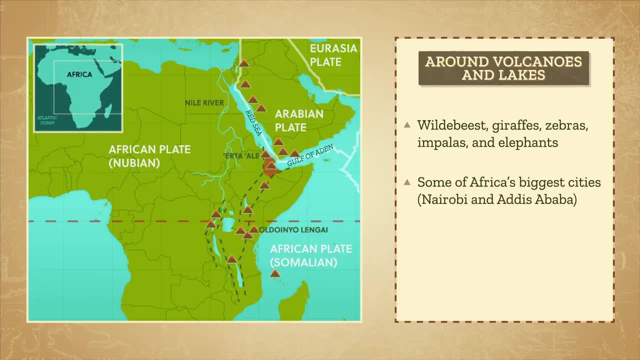 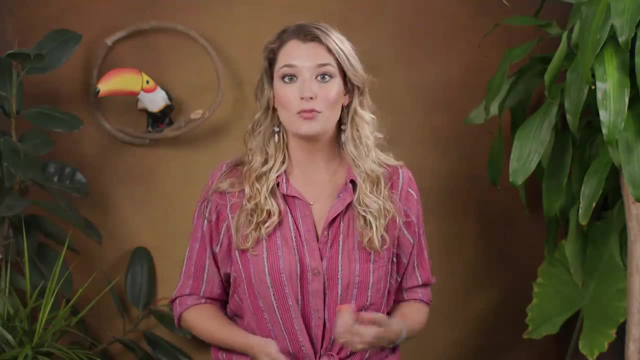 zebras, impalas and elephants, but also to some of Africa's biggest cities. There are also important agricultural production zones, exporting coffee, tea and sisal. But faulting isn't the only way the tectonic and rock cycles combine to create landforms. 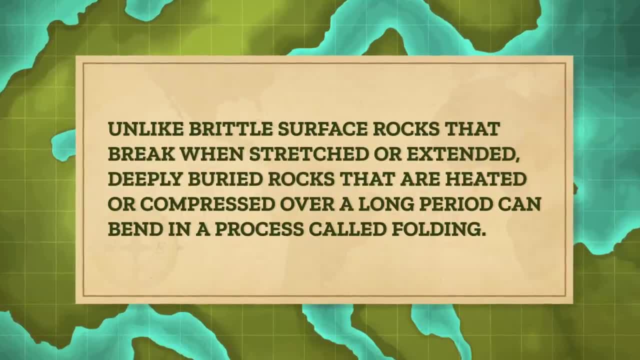 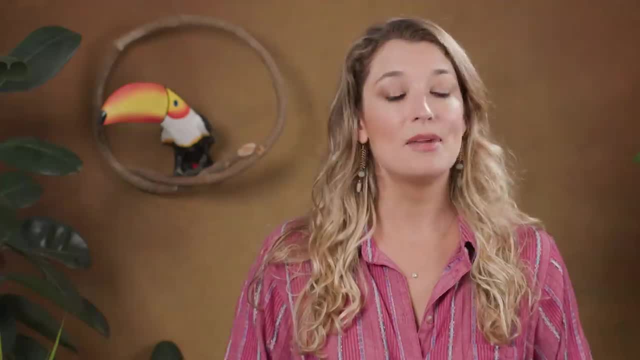 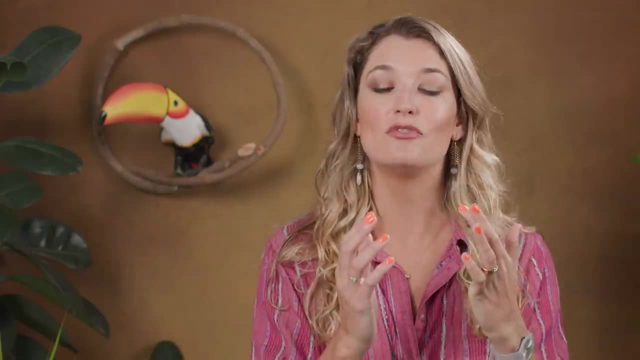 Unlike brittle surface rocks that break when stretched or extended, deeply buried rocks that are heated or compressed over a long period can bend in a process called folding. Remember, sedimentary rock forms horizontal layers or strata And when they're squeezed or compressed, like when two continental plates collide, at converging. 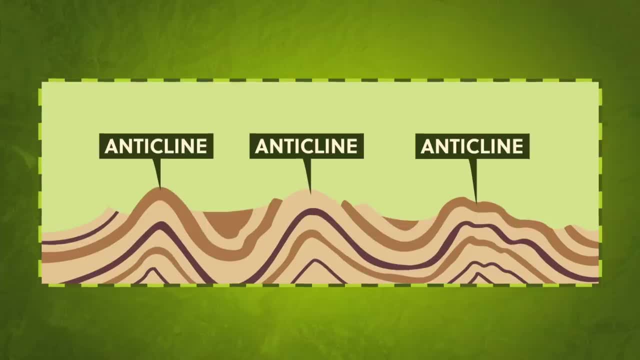 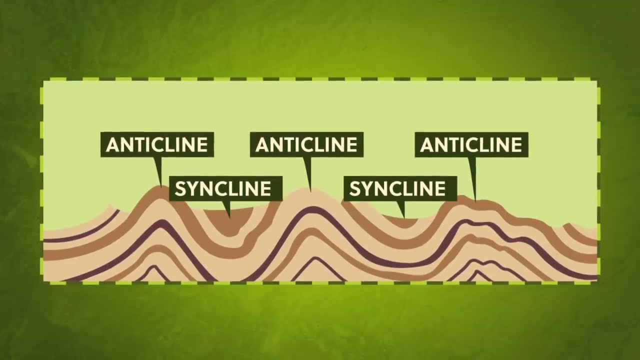 plate boundaries. they bend into arches called anticlines, which are separated by troughs called synclines. It's like if we lay out a piece of thick fabric and then suddenly bunch it together from both ends to get folds. Doing that with Earth's surface gives us foldbelts. 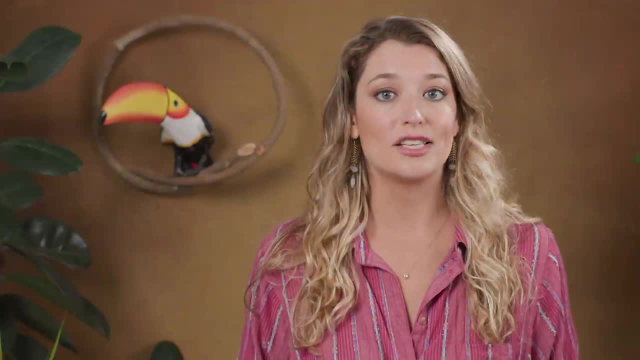 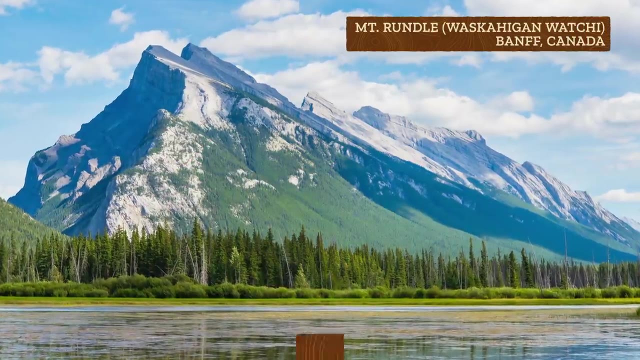 like the Jura Mountains of France and Switzerland. Both folding and faulting produce large-scale landforms and shape the landscape in really dramatic ways. Like both, can be a part of the mountain-building process called orogenesis, which literally means the birth of mountains. 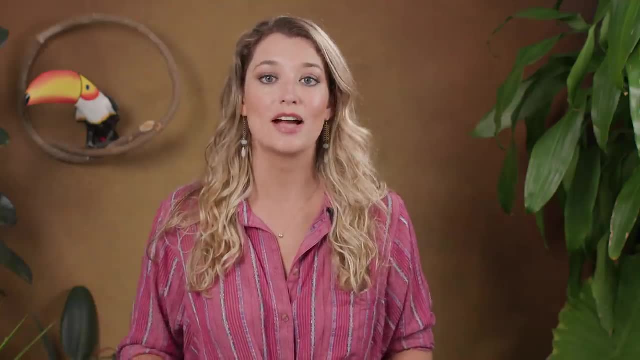 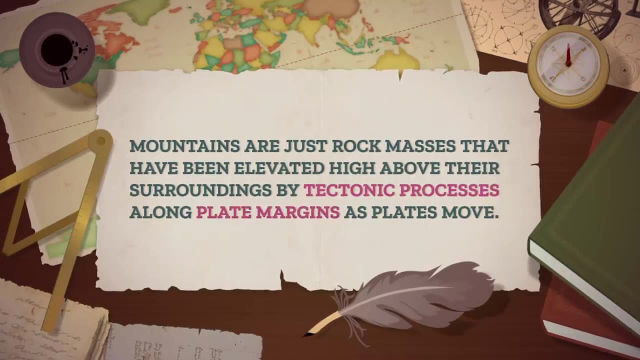 And really orogenesis is just more ways the rock cycle interacts with the tectonic cycle. Mountains are just rock masses that have been elevated high above their surroundings by tectonic processes along plate margins as plates move, Like when the Indian Plate buckled into the Eurasian Plate- vast, folded and faulted mountain. 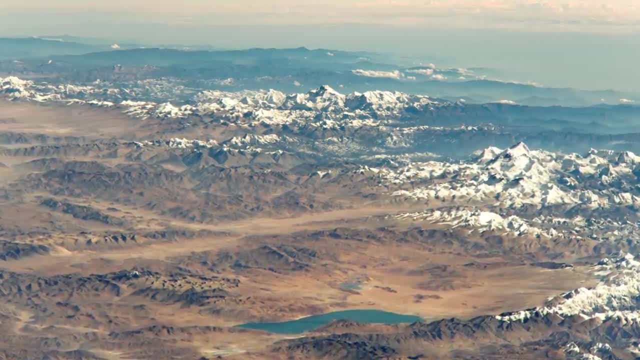 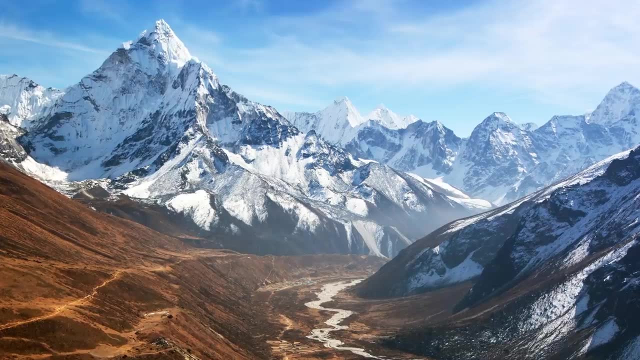 belts rose and rocks in the crust were thickened, deformed and metamorphosed. The collision created the Himalayas, which are really more like three broadly parallel ranges that each mark a different sequence in the uplift process, Processes that are still happening. 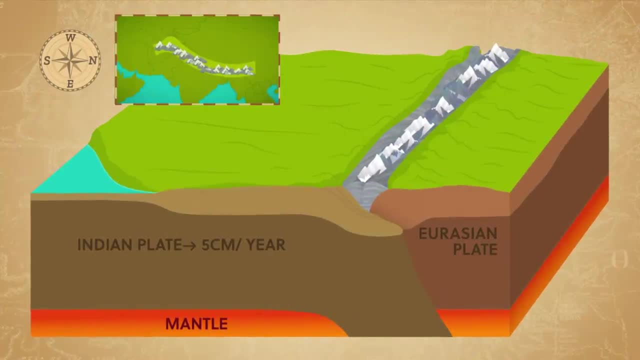 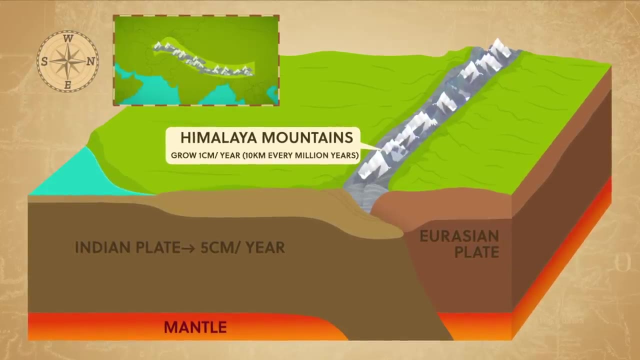 Currently, the Indian Plate pushes northward at the breakneck speed of 5 centimeters a year, causing the Himalaya Mountains to continue to grow at the rate of 1 centimeter each year, or 10 kilometers every million years, Which in geological terms, is like warp speed. 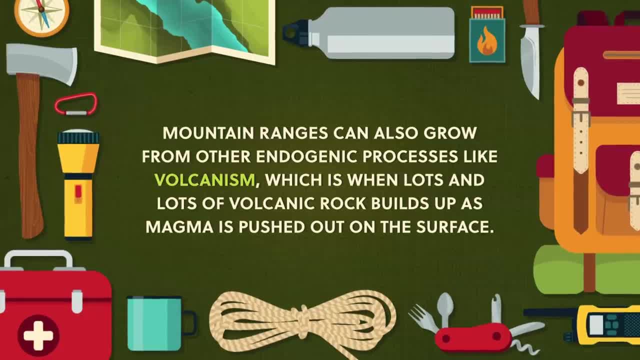 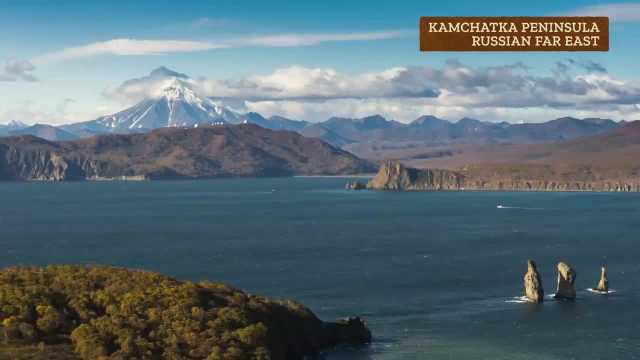 Mountain ranges can also grow from other endogenic processes like volcanism, which is when lots and lots of volcanic rock builds up as magma is pushed out on the surface, Like on the Kamchatka Peninsula in the Russian Far East, which is a dramatic volcanic landscape of immense beauty. On this relatively small bit of coastal land, there are over 300 volcanoes, of which 29 are active. The volcanoes are mountains or hills constructed from igneous processes, when magma deep within the Earth erupts onto the surface as lava and then cools and solidifies. 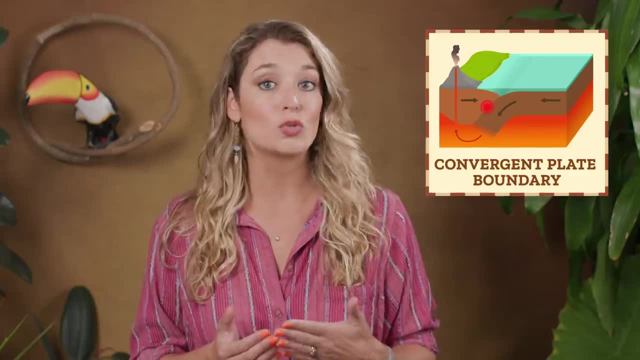 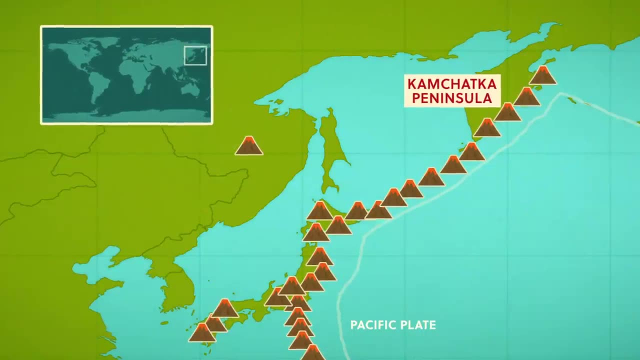 Most commonly, magma reaches the surface where two plates meet, which is why many volcanoes are located above subduction zones, where one tectonic plate is being dragged under another. Here in Russia, the Kamchatka Peninsula lies to the west of the Kuril-Kamchatka Trench. 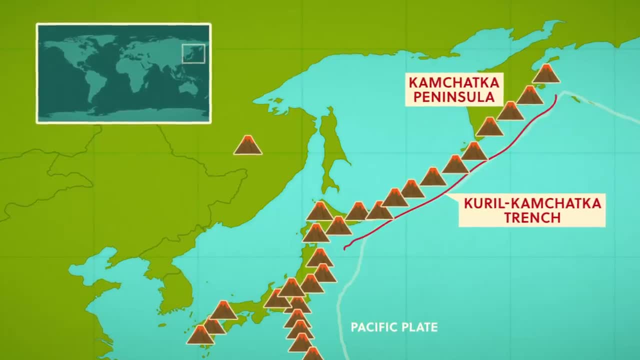 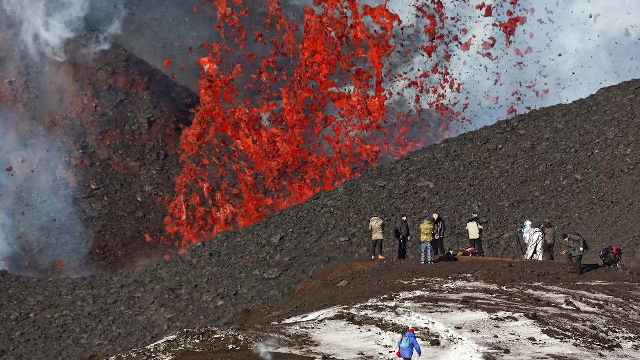 where the plunging Pacific Plate creates a subduction zone and causes volcanic activity. So when we're looking at an active volcano or any mountain, what we're really seeing is part of Earth's tectonic cycle unleashed through endogenic processes which bring fresh water to the surface. 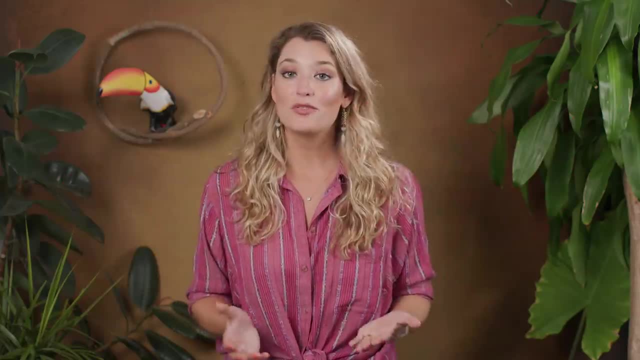 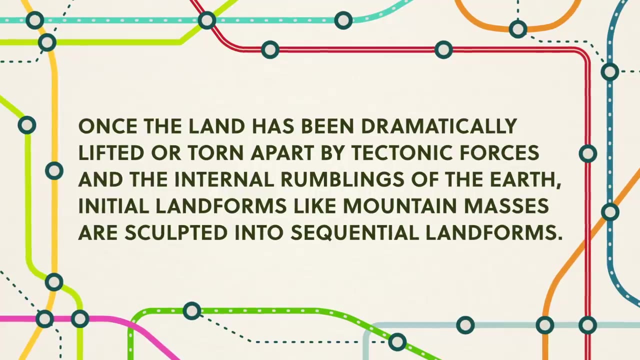 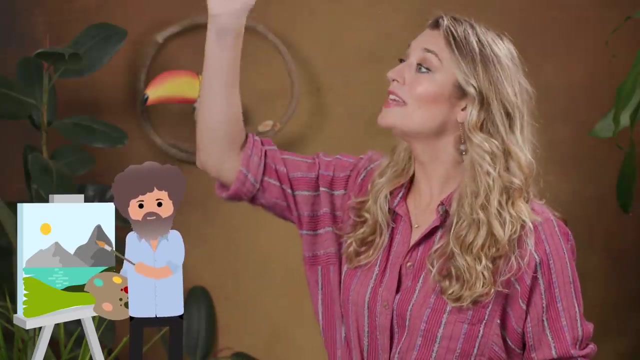 So our picture of the Earth is coming along nicely. Once the land has been dramatically lifted or torn apart by tectonic forces and the internal rumblings of the Earth, initial landforms like mountain masses are sculpted into sequential landforms. These are the details: the happy little peaks and valleys. and other features honed by external or exogenic processes acting on the surface that remove rock materials and reduce the land. In endogenic processes, the tectonic and rock cycles are the main players shaping the Earth's crust, But in exogenic processes the hydrological cycle comes into its own as it interacts with the rock. 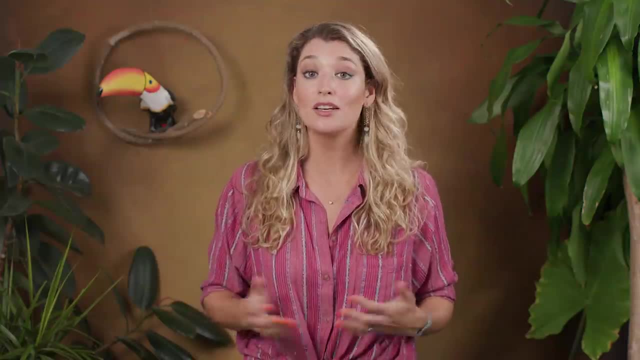 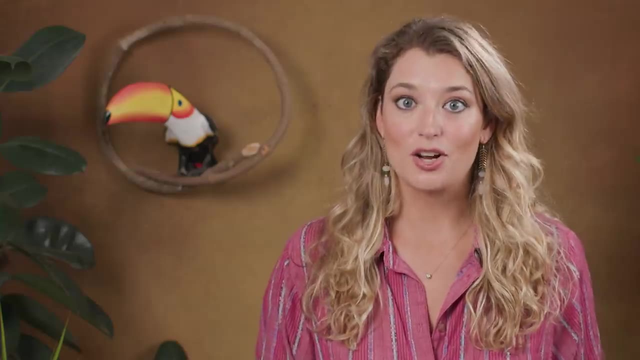 cycle. Water circulating from the ocean to the atmosphere is important in the annual march of seasons, but also in the geological cycle by which Earth renews and reproduces itself. Like the vapor in the atmosphere, comes down to produce life and growth, and create soil from rock through weathering or the decay and disintegration of rocks. 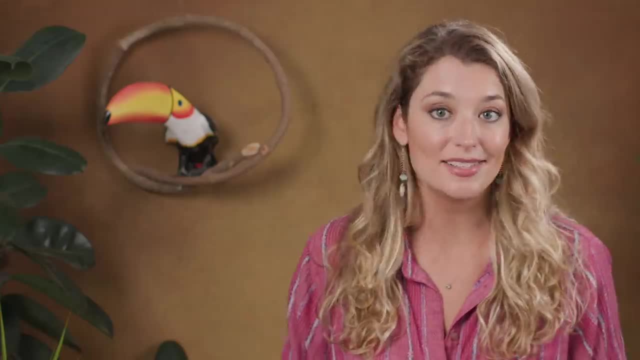 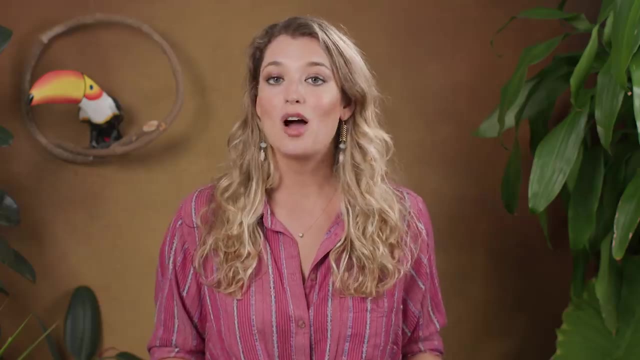 Over time, the weathered rock is picked up and carried by water, wind and ice in the process of erosion, where it accumulates to make sedimentary rock or gets subducted with the diving oceanic plate. Different rocks offer different resistance to weathering and erosion, based on everything from: 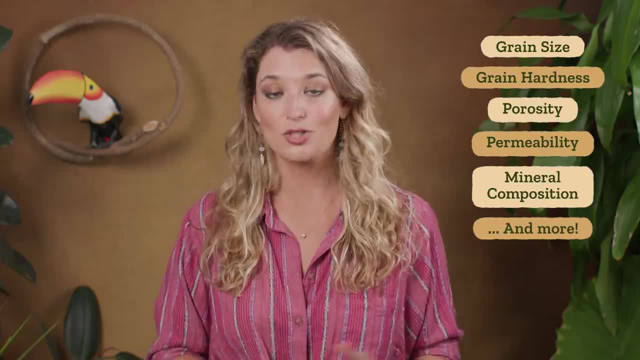 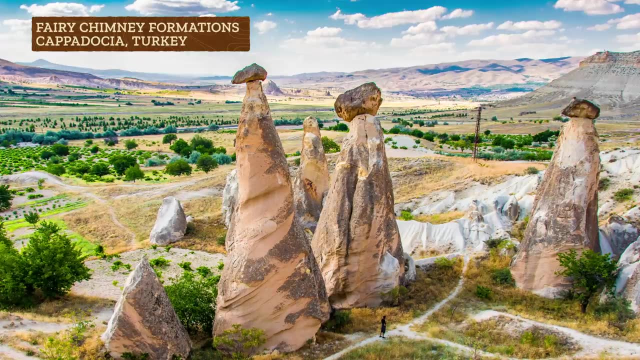 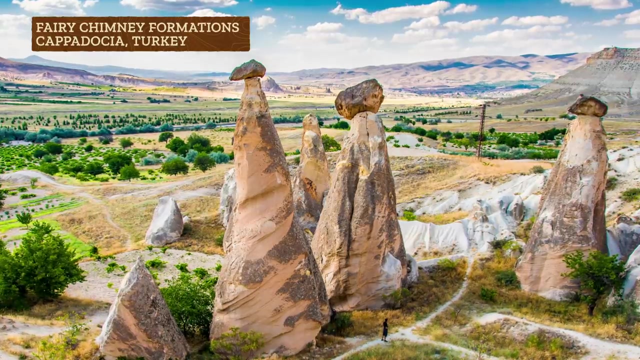 grain size and hardness to porosity and permeability to their mineral composition. But resistance actually has a big influence on how landforms and landscapes look. Rocks that are resistant to weathering and erosion will stand higher than less resistant rocks, and weathered rock is more easily picked up, moved and deposited somewhere else. 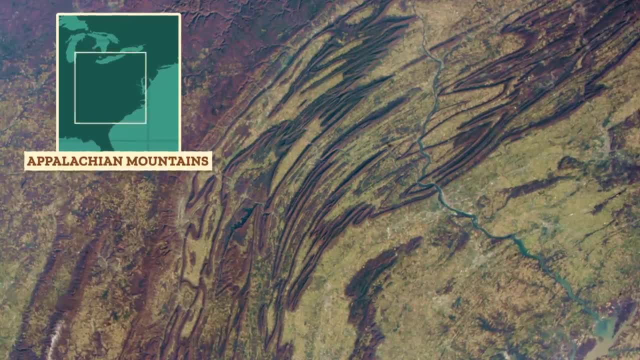 Like when folds are deeply eroded in the Appalachian Mountains along the eastern part of the US. They eventually become larger, And that is the state of the world when rocks are deposited into the Arctic, the Arctic region or the Atlantic Ocean, And it's also important that rocks are 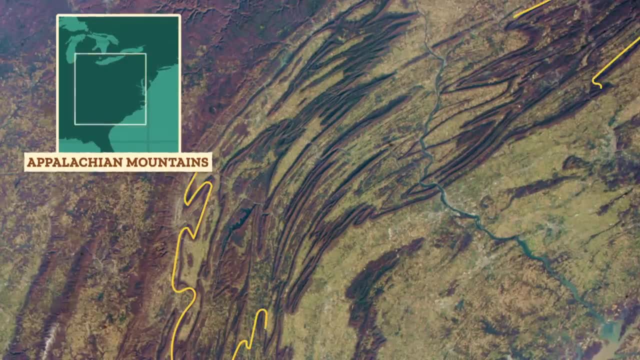 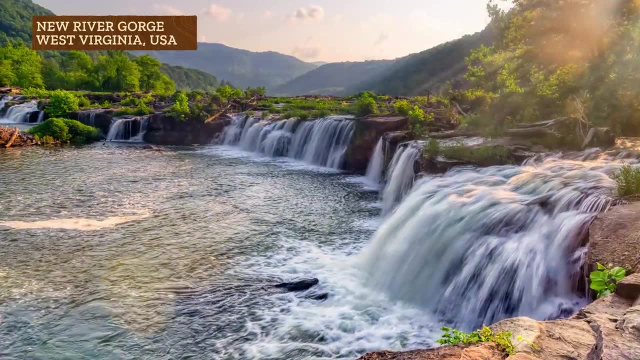 end up as ridges and valleys. As weaker rock like shale and limestone eroded, it left hard sandstone and quartzite to stand as long, narrow parallel ridges, And the ridges have been cut through and further eroded by rivers. 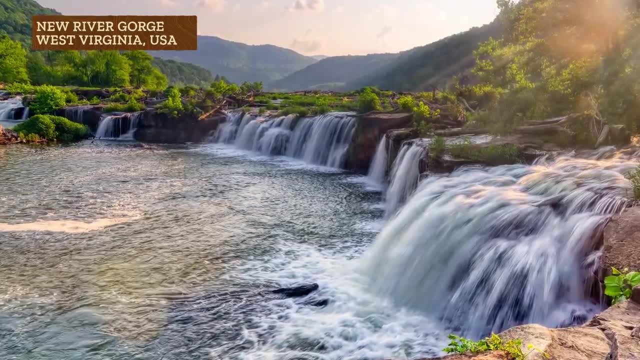 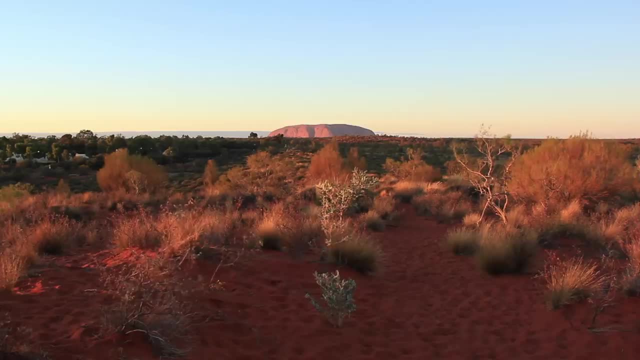 These breaks influenced migration, settlement patterns and even cultural traits in the US in the 1700s, as the flow of people, goods and ideas were guided by this topography. Weathering and erosion have also left behind some of our most stunning landscapes. 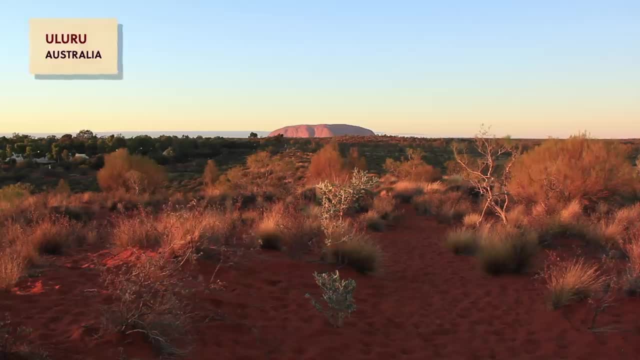 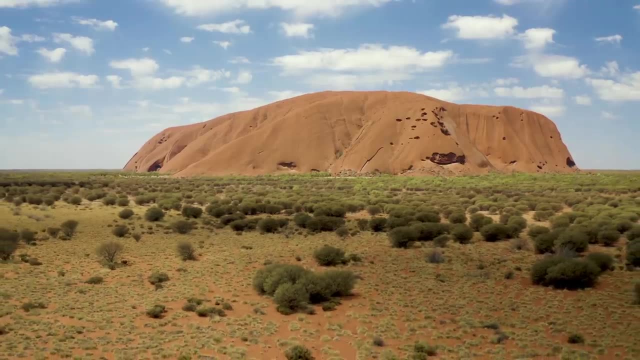 Like in the remote, dry interior of Australia's outback stands Uluru, a sandstone formation called an Inselberg that we think is 550 million years old. It looks like a 348 meter tall rock that's 9.4 kilometers around was just dropped onto. 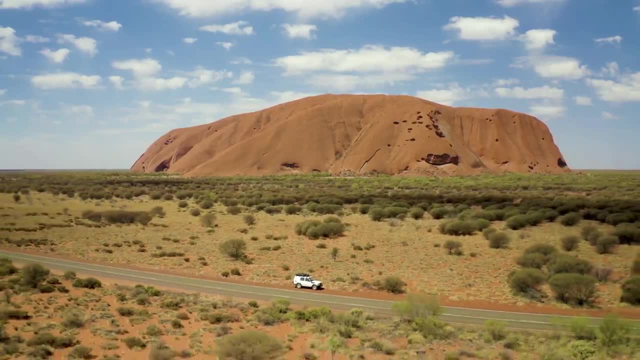 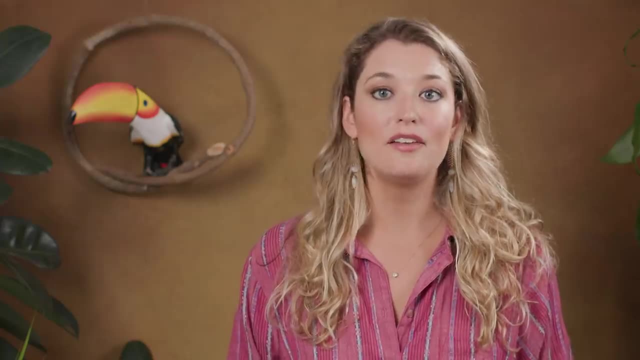 the land, But Uluru is an erosional remnant and all that remains from an ancient plain that would have been level with the present dome. Centuries of erosion by wind and water have removed the weaker rock and left erosion-resistant rock domes like this one, standing above the surrounding landscape. 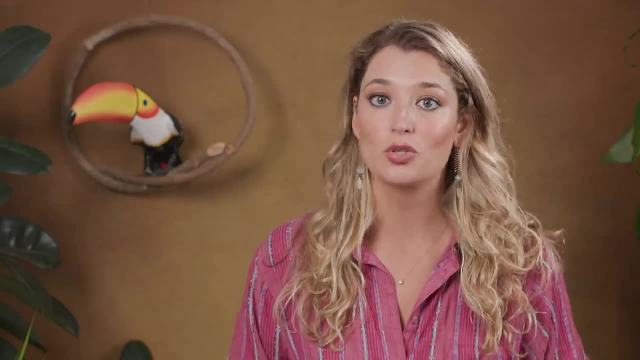 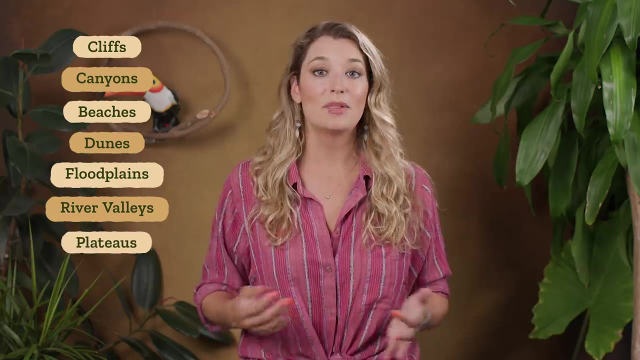 Uluru is the most famous and is sacred to the traditional landholders who have lived around the rock for thousands of years. Cliffs and canyons, beaches and dunes, floodplains and river valleys, plateaus and mountains – these are all products of a restless Earth and greatly influence how people live and 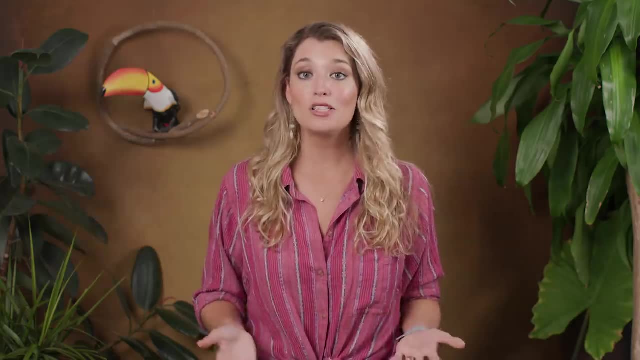 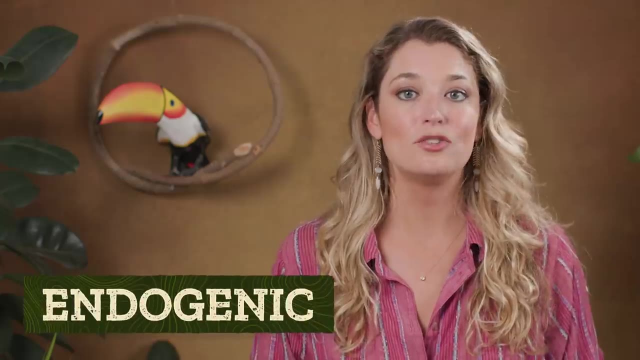 derive meaning and a sense of place in different landscapes. Ultimately, landscapes are a part of our collective human experience, our struggles and our triumphs. In the next few episodes, we'll talk more about endogenic and exogenic processes, especially weathering, erosion and the power of water, because of how fundamental they are to both. 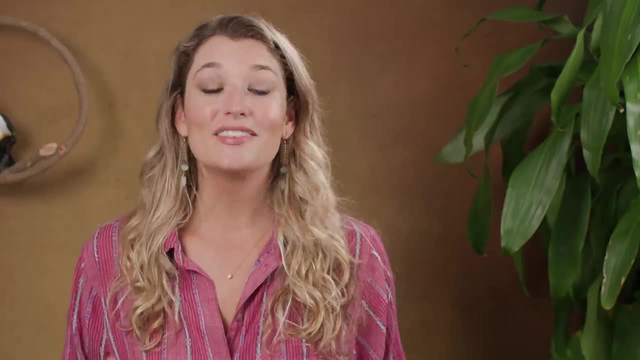 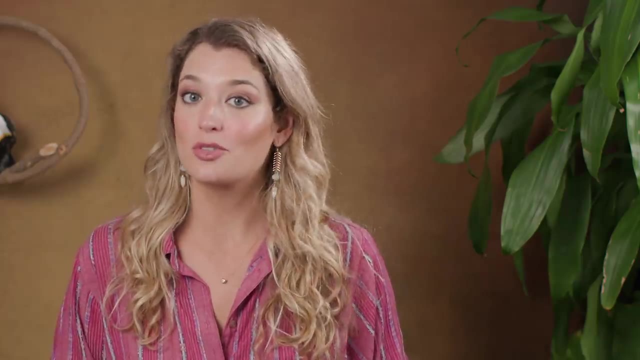 the ordinary and extraordinary landscapes around us. The Earth does change beneath our feet, sometimes infinitely slowly, as with tectonic processes, and sometimes instantly, when volcanoes erupt. Next time we will look at the grand fireworks show that nature puts up to see the different. 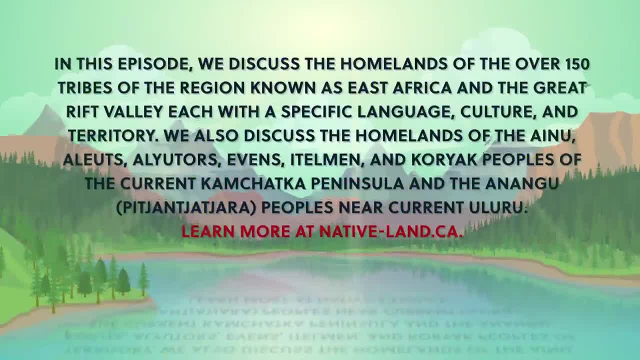 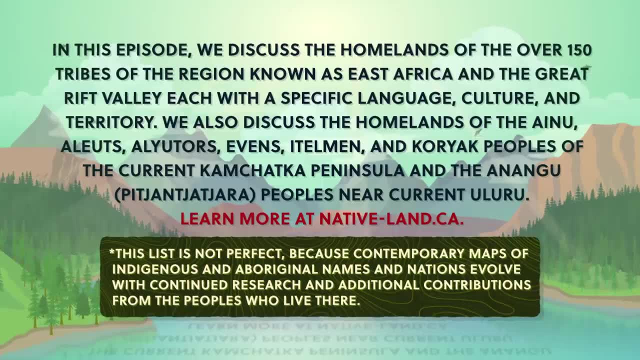 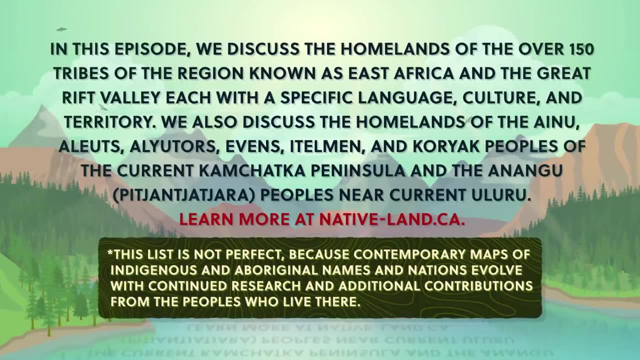 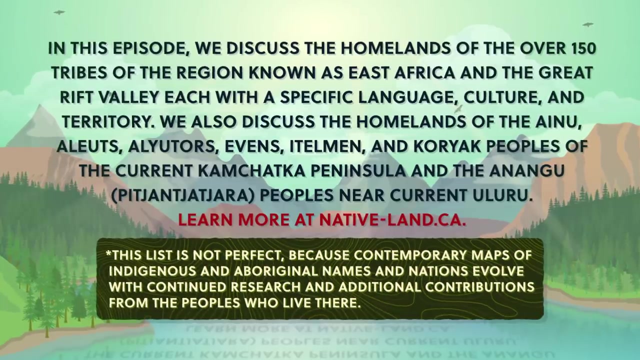 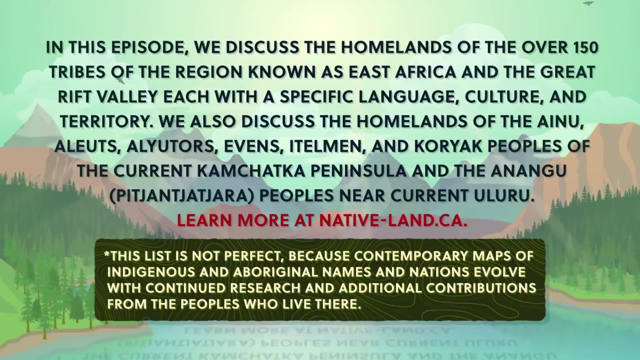 types of volcanoes and different landscapes. they produce Many maps and borders, represent modern geopolitical divisions that have often been decided without the consultation, permission or recognition of the land's original origin. So let's get started. Let's get started. Thanks for watching this episode of Crash Course Geography, which is filmed at the Team. 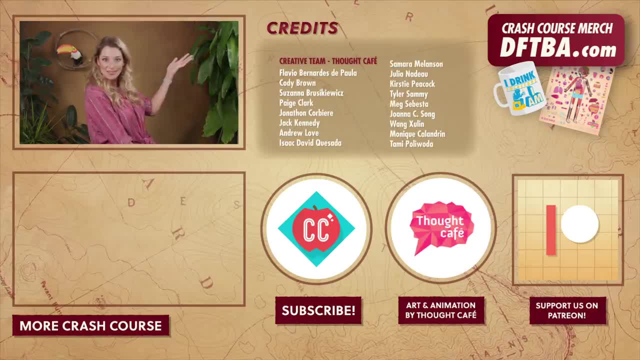 Sandoval Pier Studio and was made with the help of all these nice people. If you want to help keep Crash Course free for everyone forever, you can join our community on Patreon.